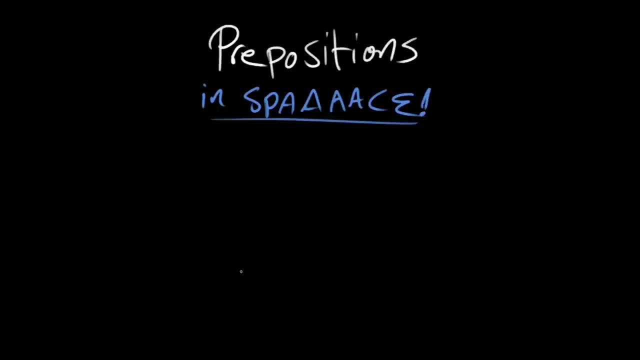 that prepositions do is they can set up relationships between objects and their locations, right? So I could say the triangle is over the square right Or on top of the square. I could say the circle is inside the square Right, and these are all so you know. 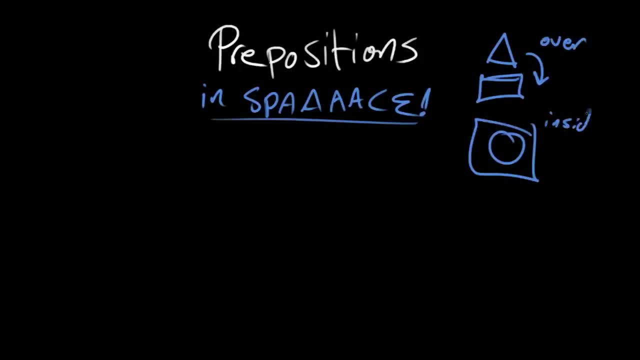 over inside. What I would like to do is review some of the major ones and talk about what their uses are. So, when we use the word at in a sentence- and here I'm talking about- something we should note is that some of these prepositions 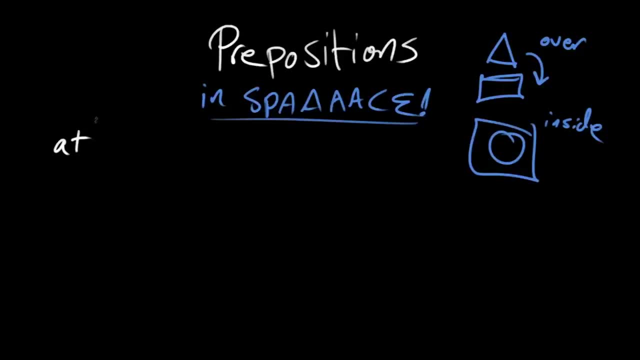 can be used in multiple ways, right? So at has a space connotation, but it also can have a time connotation. But I don't want you to really worry about that right now. I think it makes the most sense to just think of their uses. 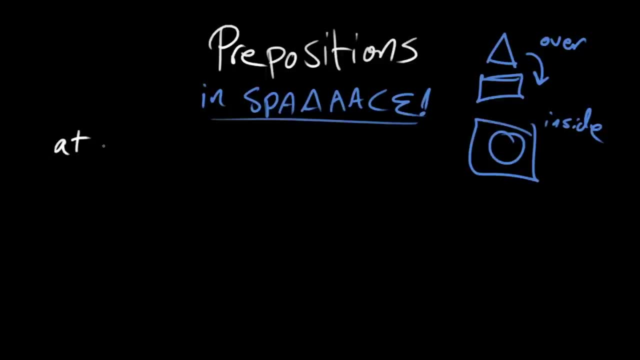 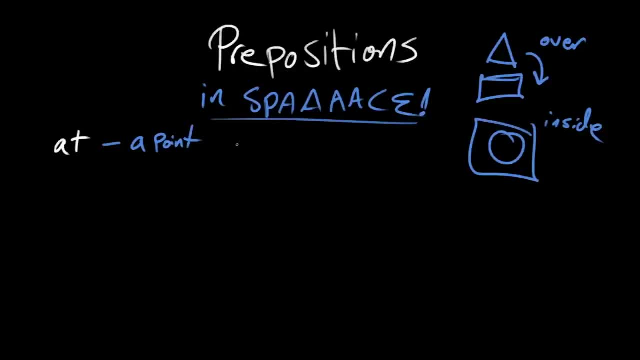 a point. right, it's talking about a point, So we could say something like we stood at the entrance to a cave, But it can also have this connotation of direction, as in the creature launched itself at Amina. The word by when we're talking about space. 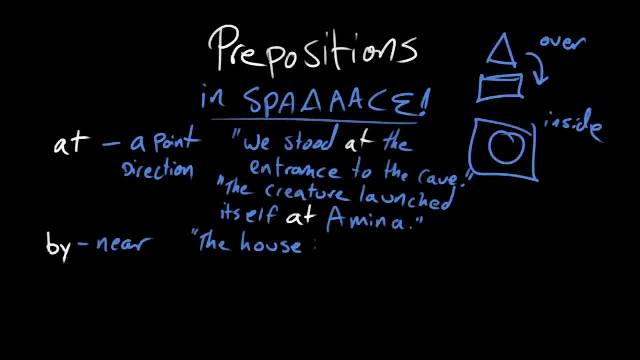 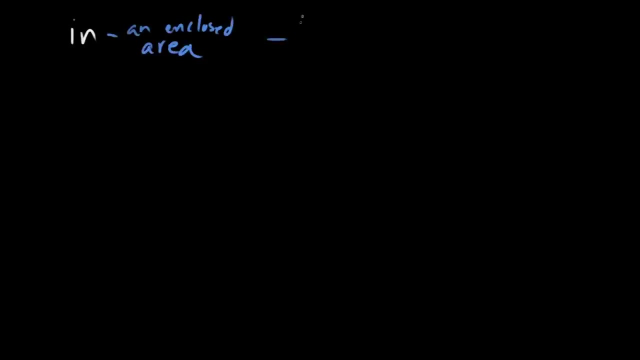 means near, as in the house by the old mill is totally haunted man. all these sentences are like really spooky. the preposition from has this connotation of coming from somewhere else to here, as in we came from Mars. in denotes an enclosed area, so you could say something like: 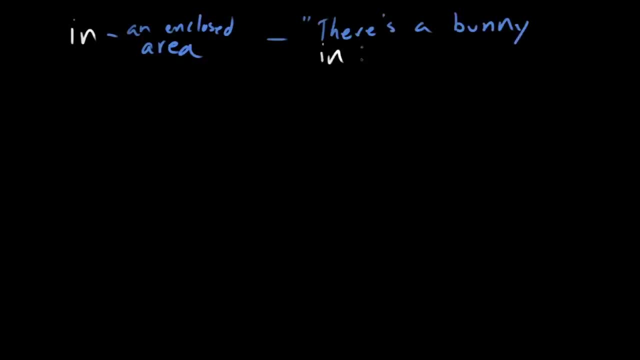 there's a bunny in the box off denotes you know away from she hopped off the rock on which you know didn't usually notes being on a surface as opposed to in which is in an enclosed area, right, like I said, so we could say there's a goblin. 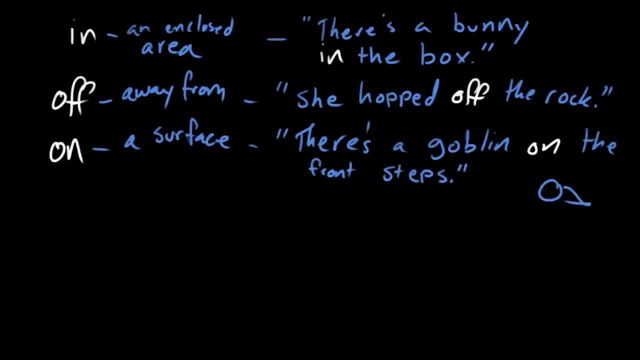 on the front steps. right, the goblin is on the steps, the bunny is in the box. see the difference. out is another direction word you know away from something. right and off, and on and in and out mean the opposite of each other. so away from out means away from an enclosed area and off. 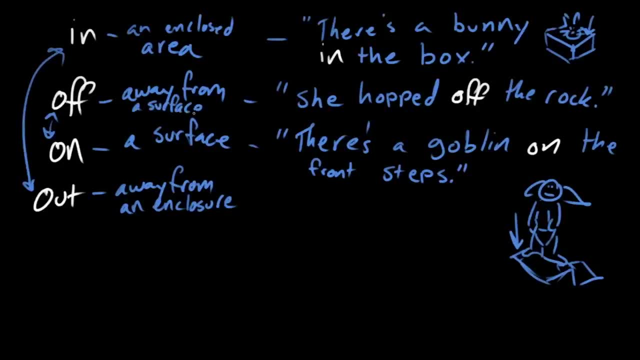 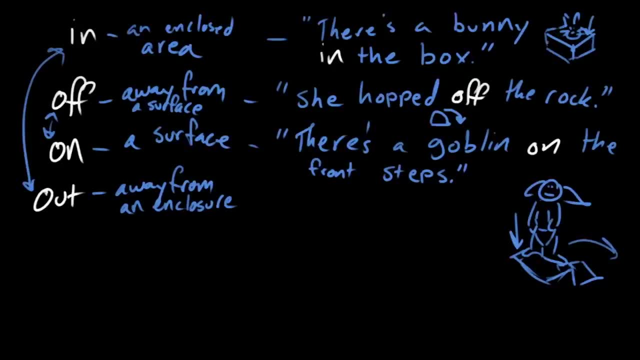 maybe the goblin leaves the front steps. he's off the front steps. there's a bunny in the box. if the bunny leaves the box, it will go out of the box. and there's plenty of other prepositions, but let's let's talk about two which, when you're 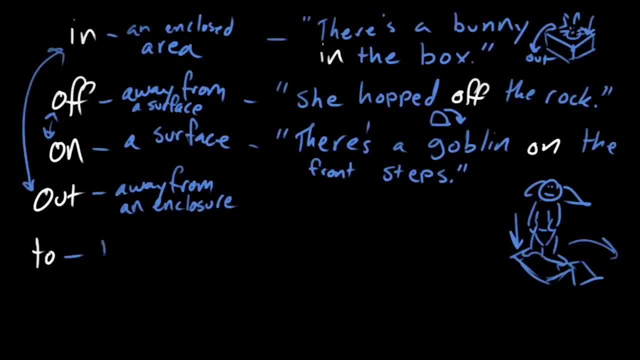 talking about two. in the physical sense it has this connotation of direction, so you could say I'm going to Mozambique. these are some of, but certainly not all of, the spatial prepositions of English. now we're lucky because prepositions are a closed group in English, a closed group. we don't. we don't add many of them to the language. 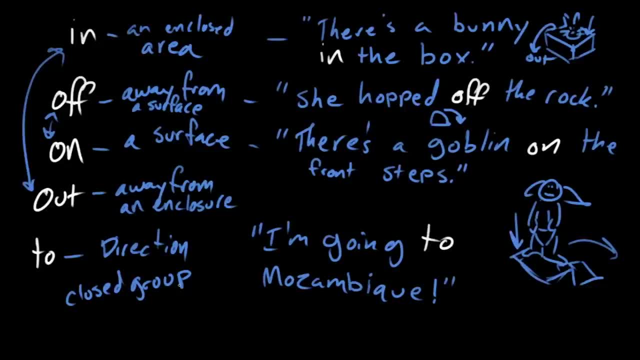 the way that we add nouns and adverbs and verbs and adjectives. there are a lot of them and you have to memorize all of them and their various obnoxious nuances. but there isn't a limitless number of prepositions. there's, you know, maybe a hundred plus and of